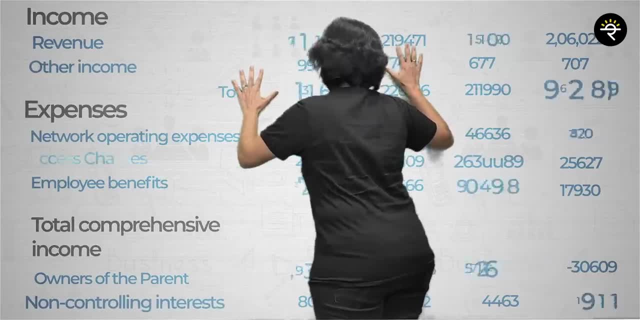 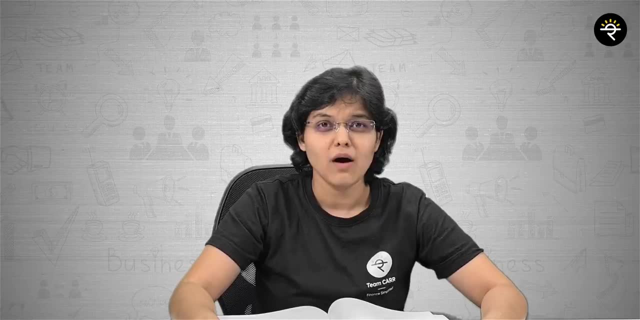 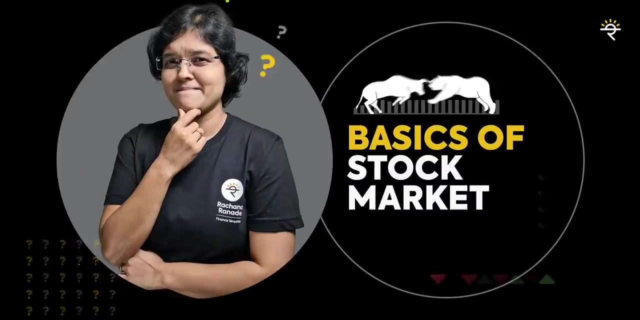 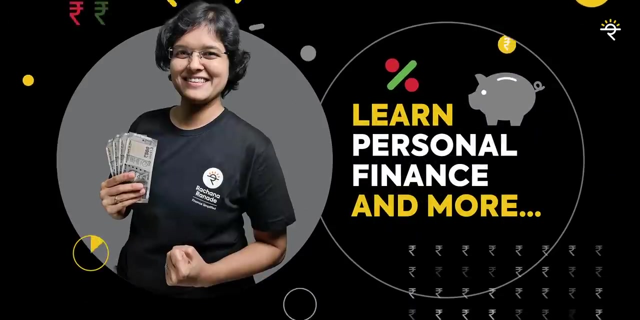 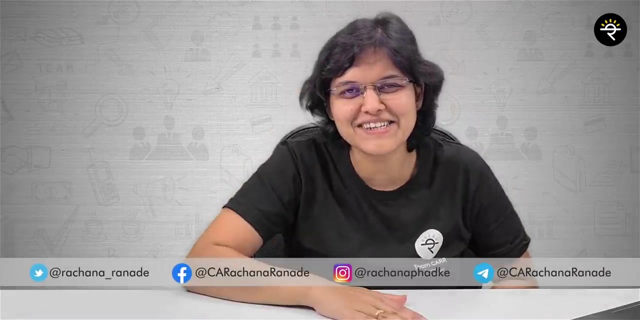 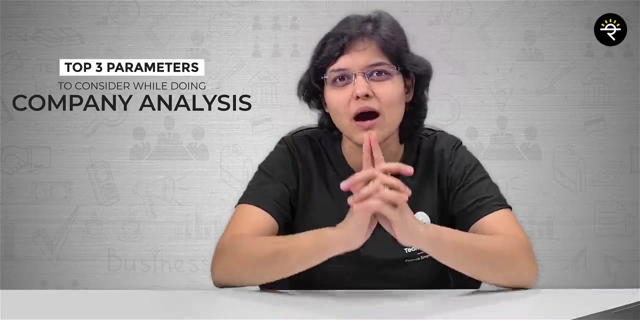 Out of all these numbers? what shall I exactly analyze? Hi guys, CA Rachana Ranade here and I welcome you all to another lecture on top three parameters that you have to do. you have to check while doing company analysis. Now, where does this? 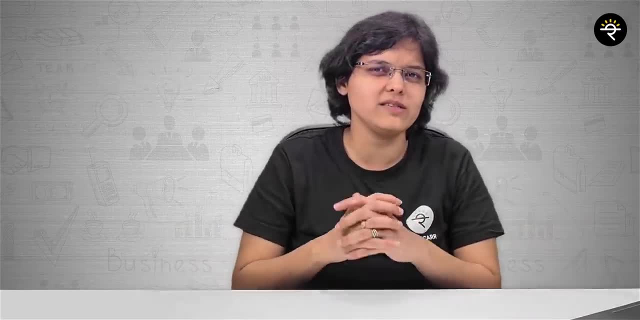 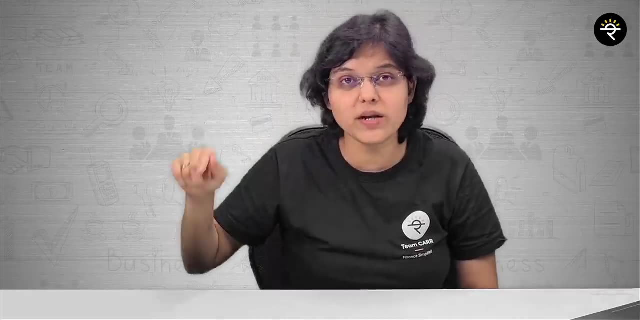 company analysis come from. It comes from fundamental analysis. So, just in case, if you don't know what all is a part of fundamental analysis, there are three major points, and which are these three? The very first one is economy analysis, next one is industry analysis and the 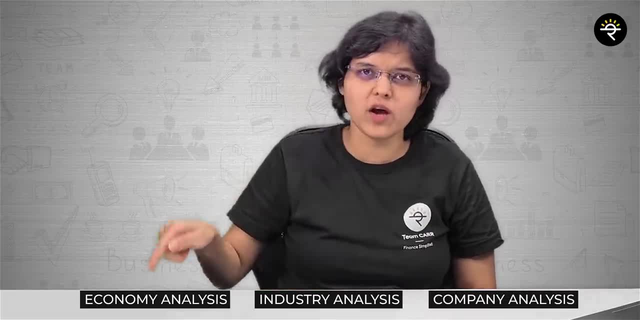 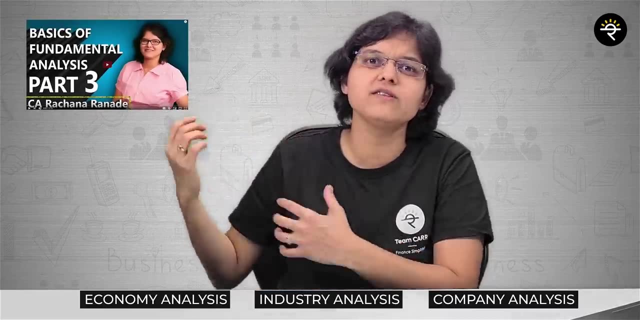 last one is company analysis. Okay, now, if I'm talking about these first two, economy analysis, industry analysis- for this you can check out my video, which I've already done on YouTube, but that video has not got a lot of relevance for today's video, so you can watch that later. 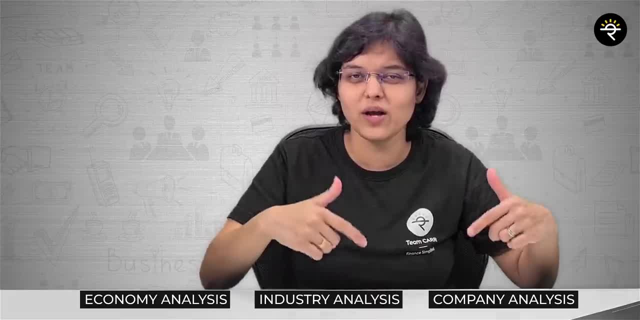 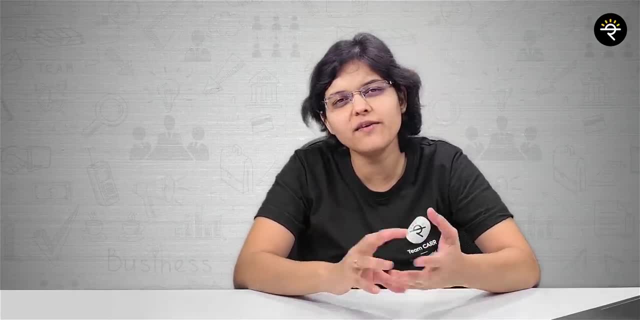 First, let us focus on top three parameters to be used while doing company analysis. So we are going to discuss about three important parameters. Does this mean that we have to check only these three parameters? Answer is obviously no, but these are at least the three basic. 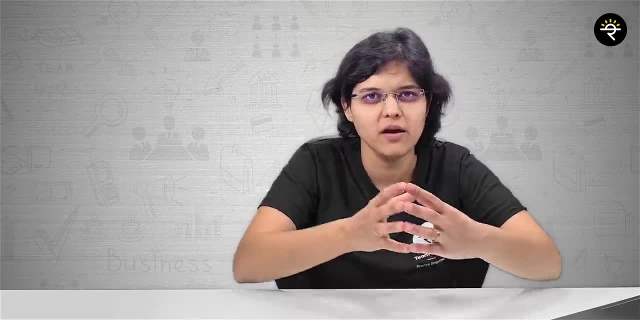 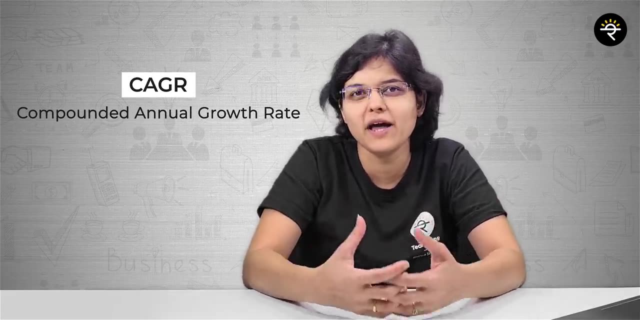 parameters that you should be checking while selecting any company for your investment. Okay, what is the first parameter? First parameter is how much CAGR, that is, how much is compounded annual growth rate for three factors. Okay, now, if you are again not aware about what is CAGR, 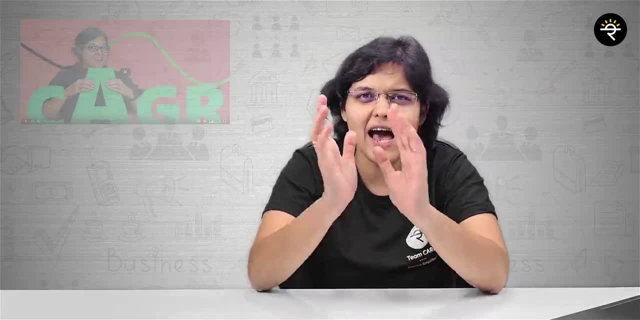 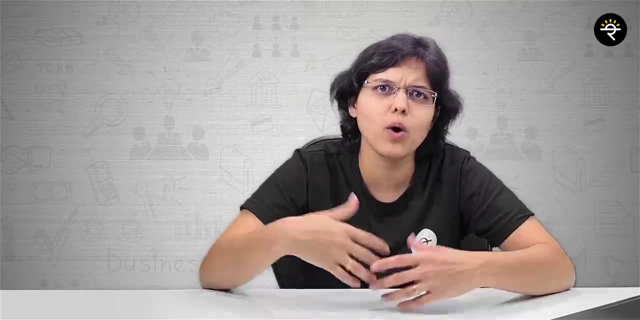 there is another video that I've done, but you can watch that later. As of now, a simple understanding: CAGR is nothing but how much growth a specific number has seen. Now what could be the number? Number could be top line- that is sales. number could be bottom line- that is your profits. 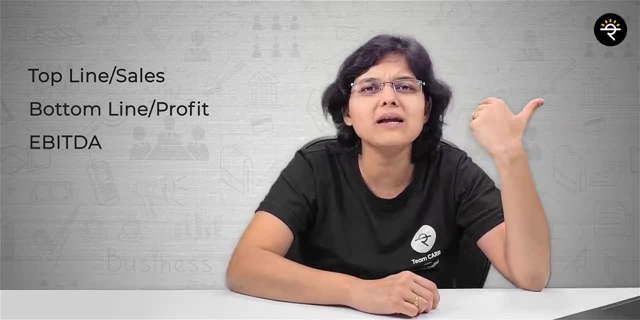 or number could be EBITDA. Okay, number could be EBITDA, that is, your profits. or number could be EBITDA. There are multiple numbers that you can get in the P&L. We are going to focus on these three. 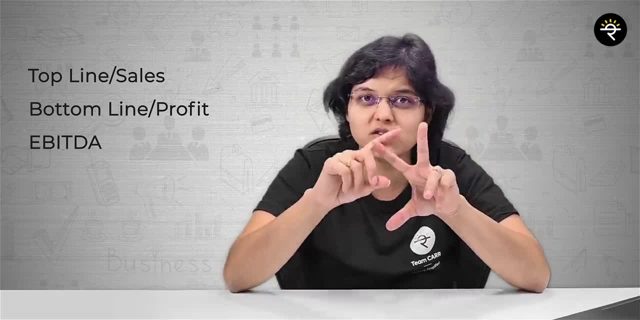 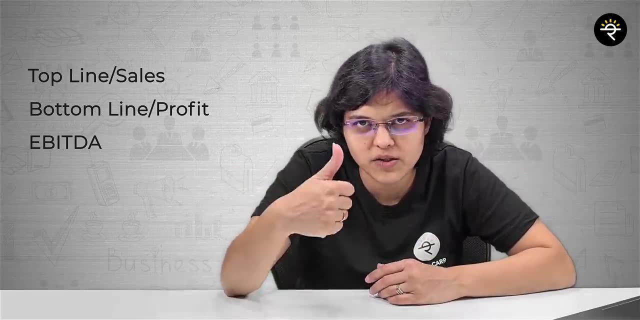 numbers. We are going to check the CAGR of sales, CAGR of EBITDA and CAGR of PAT. If all these three give a good growth, it definitely is a positive indicator. Now, why, If let us say the three years? 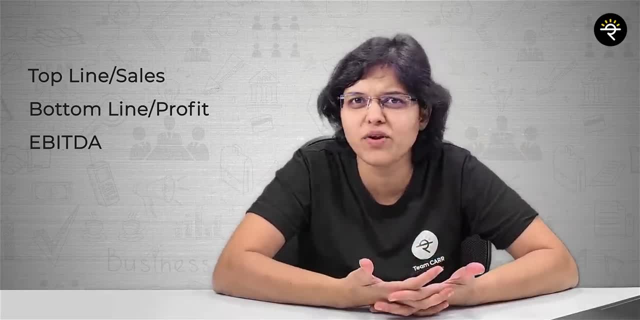 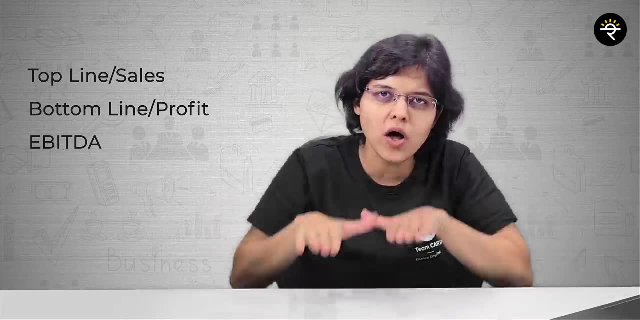 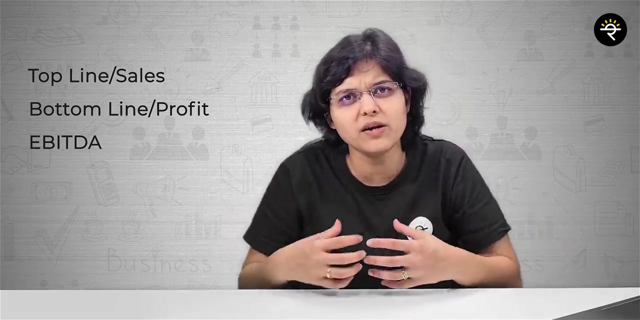 sales growth CAGR is, let us say, around 15 percent, 20 percent. what does it mean If three years CAGR for sales is 20 percent? it means that on an average, the company's sales are growing by 20 percent. Okay, similarly quick example, if the profit three-year profit CAGR is, let us say, 12, 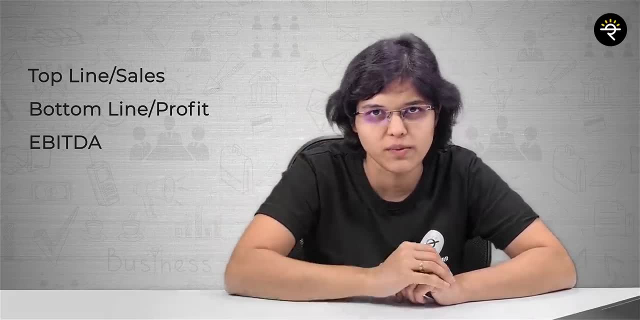 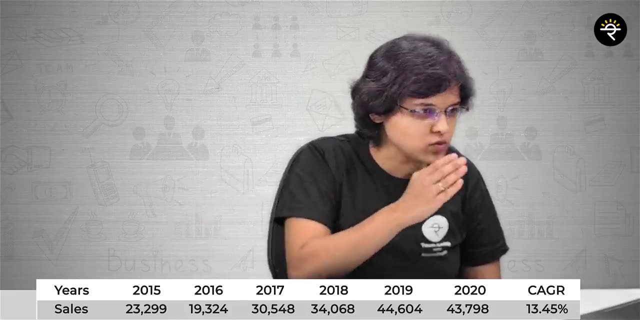 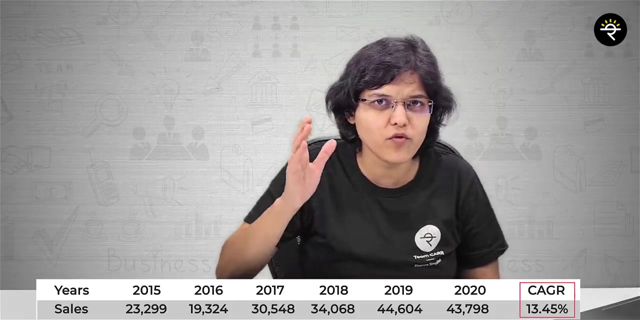 percent, it means that on an average, the company's profit is growing by 12 percent. Okay, here is a simple example of sales CAGR. You can see that the data is from 2015 to 2020 and if you just check out, if you compute what is the CAGR for all these years, it comes to 13.45 percent. Now, if 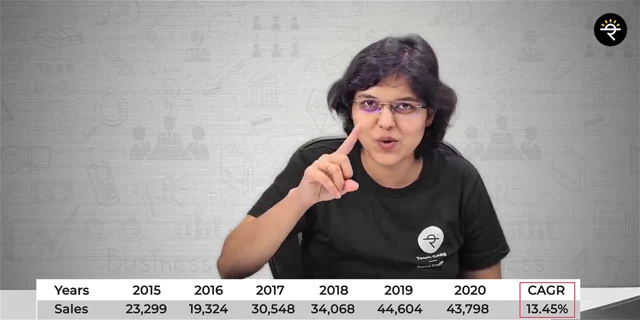 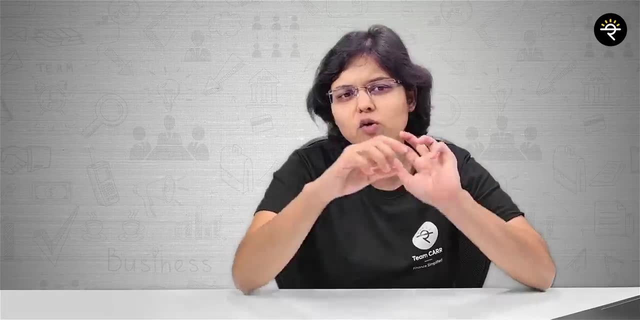 you're asking me how it means that you have not watched that CAGR video. So you can watch that video, compute and cross-check your answer. your answer has to be 13.45 percent. Okay, now one more important point. I told you three parameters to be checked. Think and give me the correct answer. 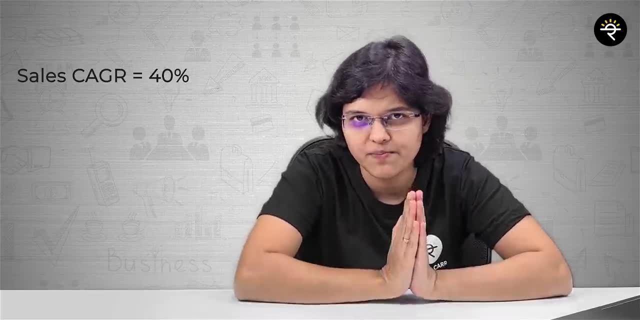 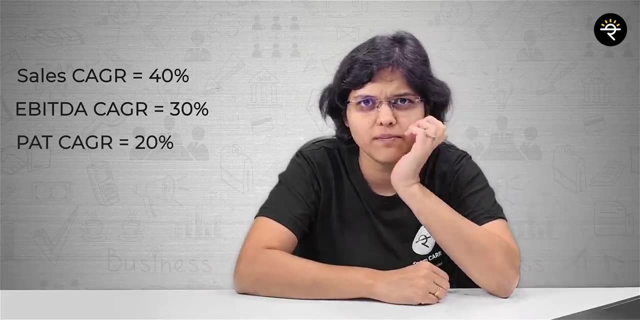 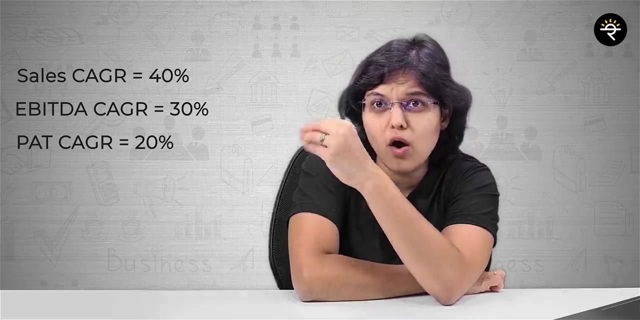 Let's say, sales CAGR is 40 percent, EBITDA CAGR is 30 percent and PAT CAGR is 20 percent. Okay, all these figures you can see here on the screen so that it will be visually very effective for you. What does this mean? Sales is growing on an average. let us say three years data again. 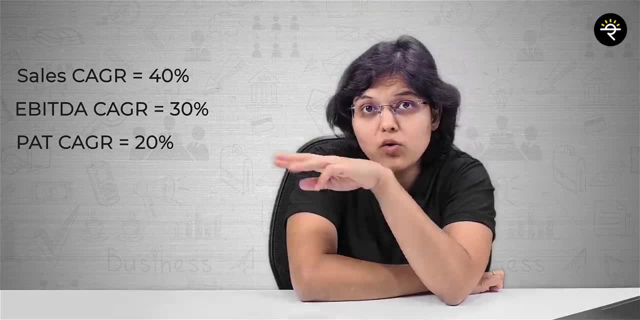 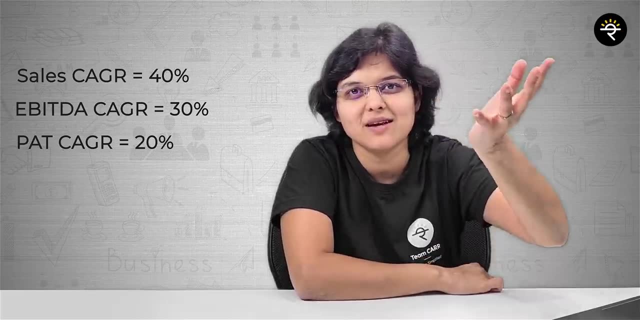 at a rate of 40 percent. So, on an average, sales grew at 40 percent, but EBITDA grew only at 30 percent. How is this possible? Why could this be possible? Could there be a possibility that the operating expenses grew at a rate higher than the revenue? So revenue is growing at 40 percent. 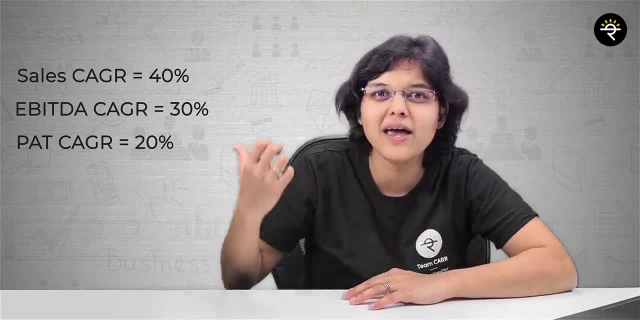 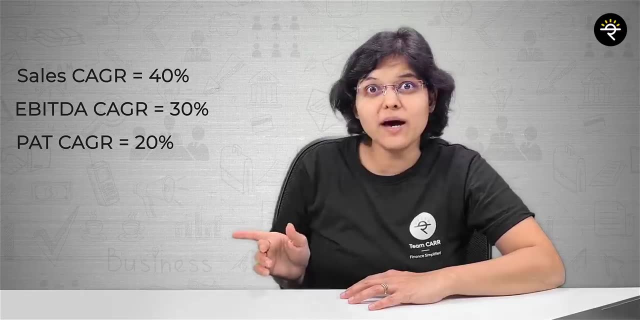 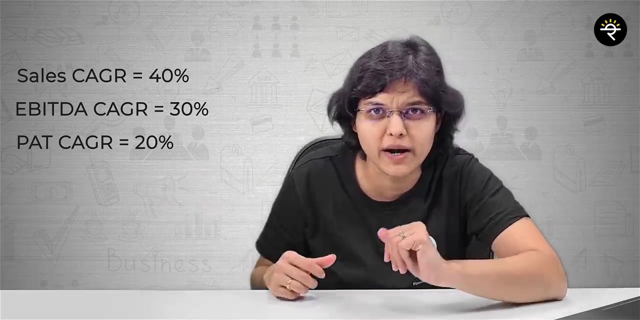 but expenses grew by, let us say, 50 percent, and that is the reason why EBITDA, your earnings grew, but grew at a lower rate of 30 percent. Okay, now your PAT margin is showing a CAGR of only 20 percent. See stand-alone. I can say 20 percent PAT growth is not that bad, But if I am comparing, 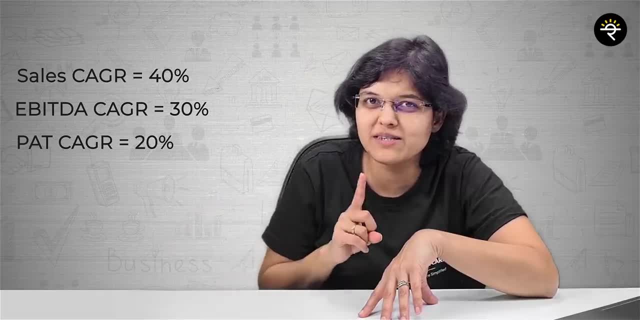 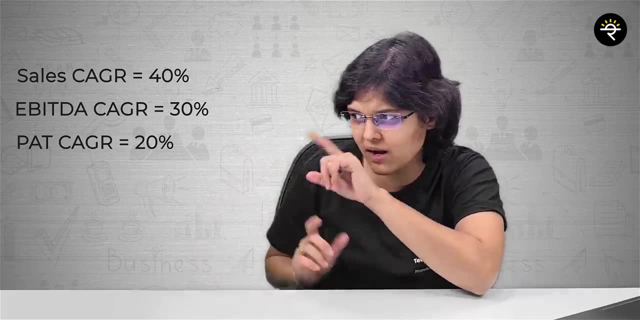 that sales is growing at 40, PAT is growing only at 20, it means that your expenses are not being controlled very nicely. and if I am talking about EBITDA versus PAT relations specifically, there could be two major expenses. either interest is growing at a very high pace or depreciation is. 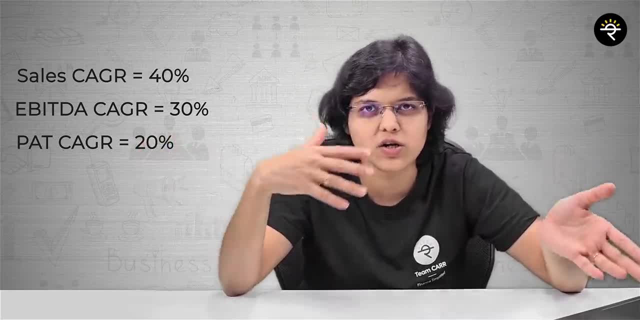 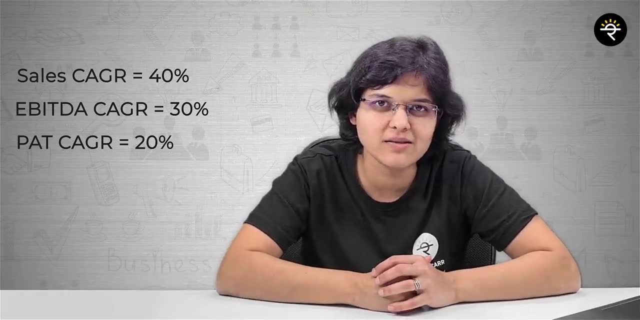 going at a high pace, So depreciation is anyways. non-cash expenditure is not a big problem, but interest is growing at a very high pace, because of which your PAT is, you see, at another level. If an dropping it means that somewhere your debt has increased and with that comes an important ratio. 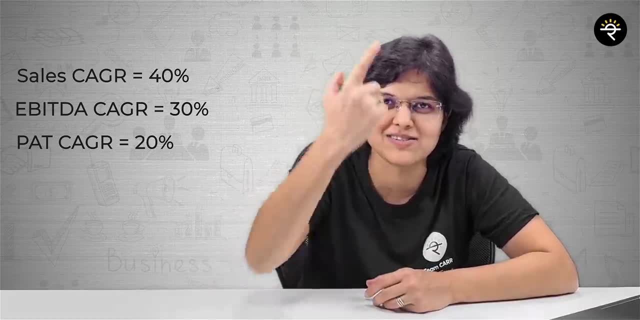 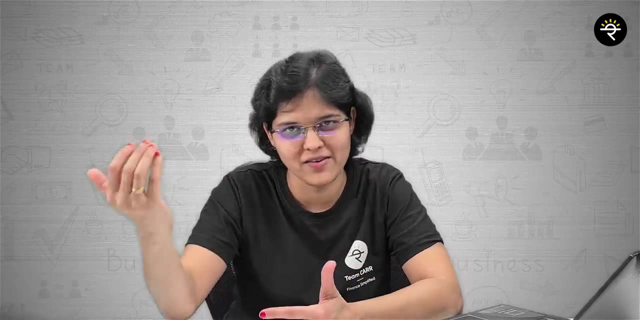 that is, debt to equity ratio, which we are going to check in the immediate next section. so if you want to start investing in shares, you definitely need a demat account and a trading account. while i was going through various comments on my channel, i came across so many comments which 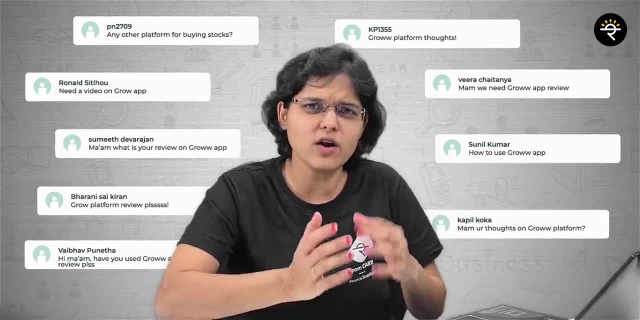 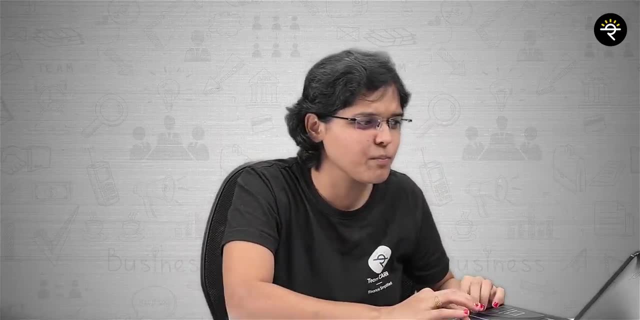 asked me about my review about the grow app, so i thought of just going through that app and i thought of sharing my views about that number one. i felt that the user interface is like pretty user friendly. so i'll just give you a simple example of what i mean. let us say i'm going through that app. 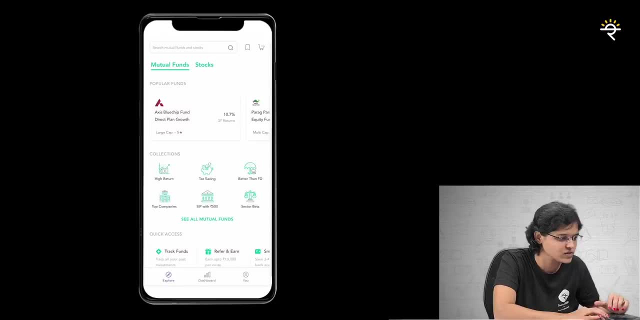 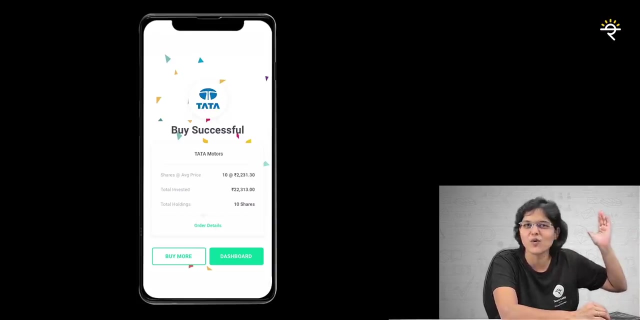 and i want to buy, just as an example, shares of tata motors. so i click here. by the way, you can see top gainers on the screen. i saw tata motors. i just click on buy tab. once i click on buy tab, i just have to input how much quantity i want. market price is there, i hit buy and yes, that's how the 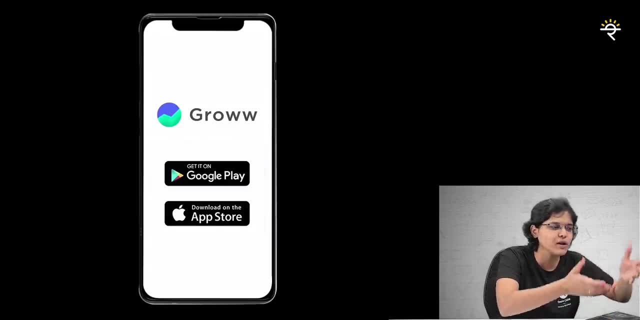 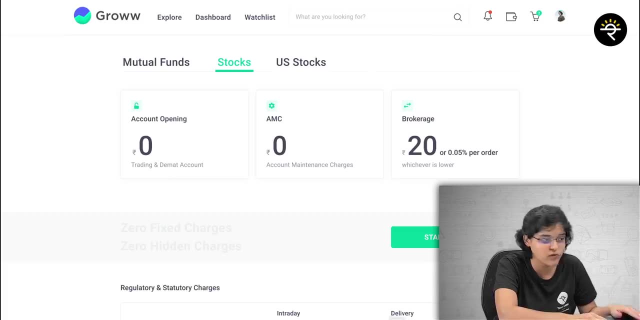 buy order is successful right away. so it's a pretty simple user interface. so if you want to talk about their pricing part uh, two, three points. i would like to highlight number one: account opening is absolutely free of cost. the amc, which is annual maintenance charges, are also free of cost. brokerage is 20 rupees or 0.05. 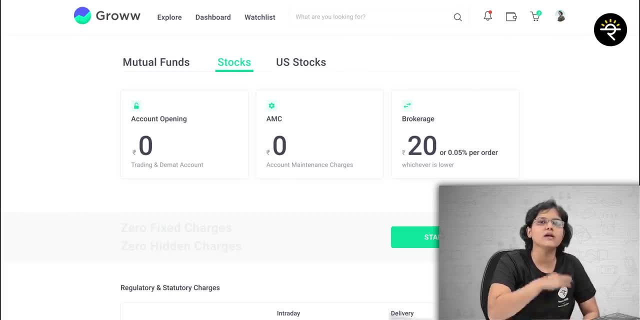 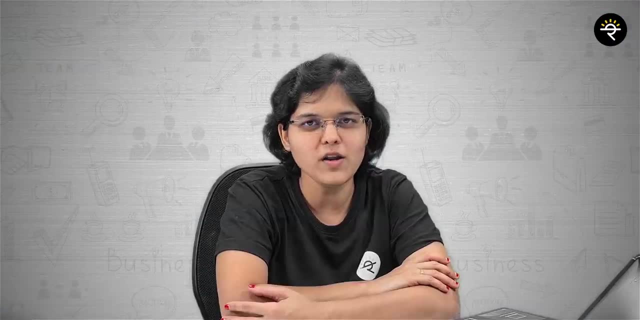 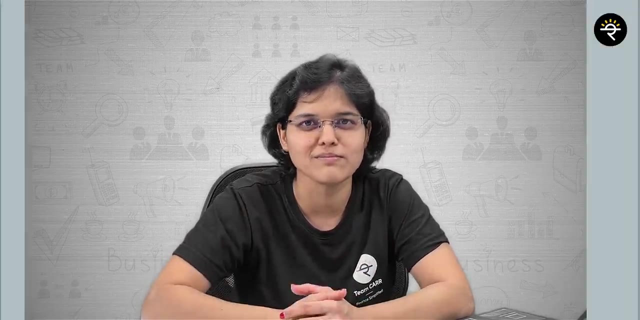 percent per executed order. just in case, if you want to check the pricing more in detail, i have put the pricing link and account opening link in the description box. well, all in all, i feel that it's always a good idea to invest in stocks, mutual fund, gold, all with the help of a single platform. now, with the basic point of debt to equity ratio, let's 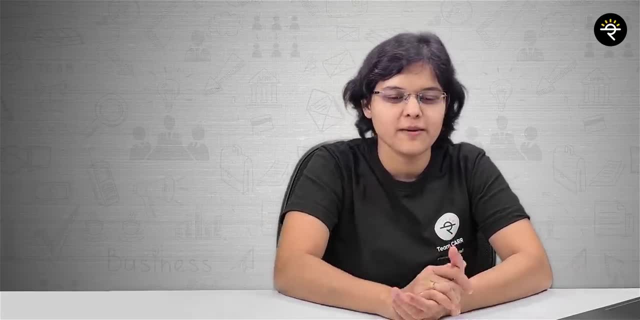 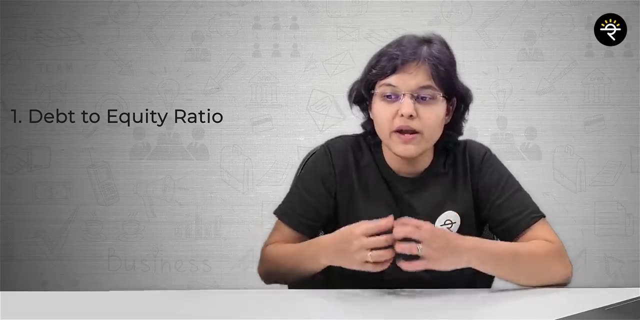 understand what could be the three important ratios that you have to check. the first one that, as i was mentioning, is the debt to equity ratio. now, what is debt? that is nothing but the borrowing. how much money does the company owe? and if i'm talking about equity, equity is owners funds. so 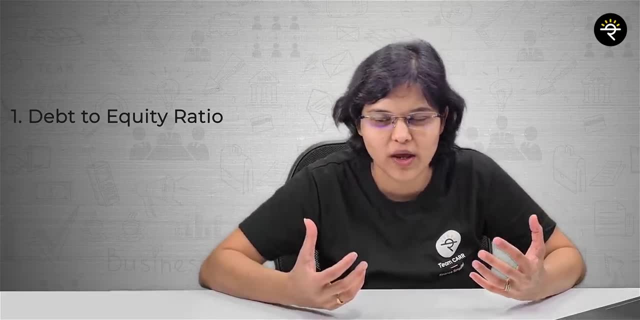 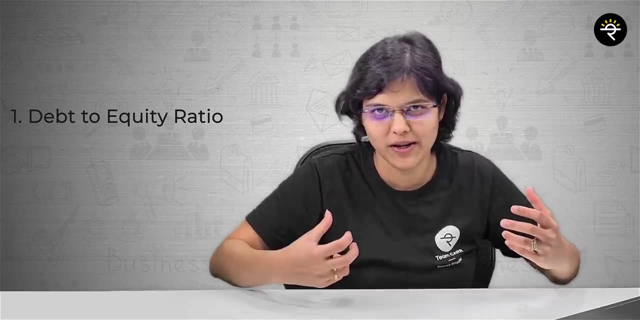 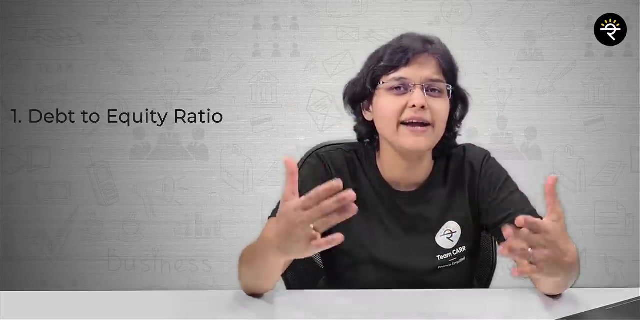 it's basically a loan. funds is to own funds ratio. okay, so how much loan should i be taking? in comparison with the own funds is nothing but your debt to equity ratio. so it is said, as per the standard financial management terminology, that your maximum debt to equity ratio, or the ideal. 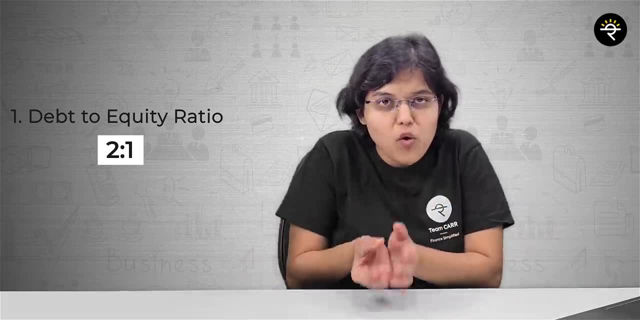 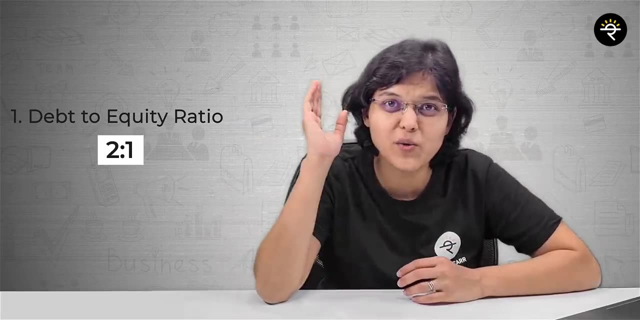 debt to equity ratio should be. two is to one means what? one rupee of own funds? if i'm putting in the business, then two rupees should be from the loan funds as on a higher side, not more than that if your debt to equity is like crazy. twenty two is to one or something. 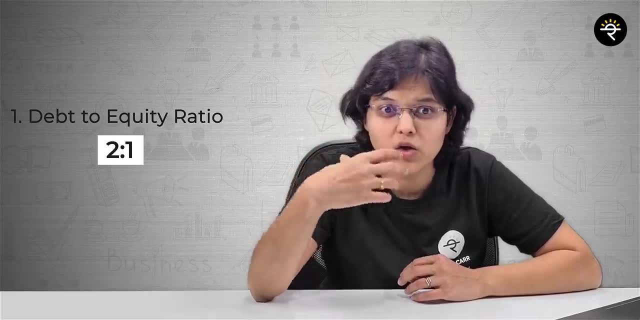 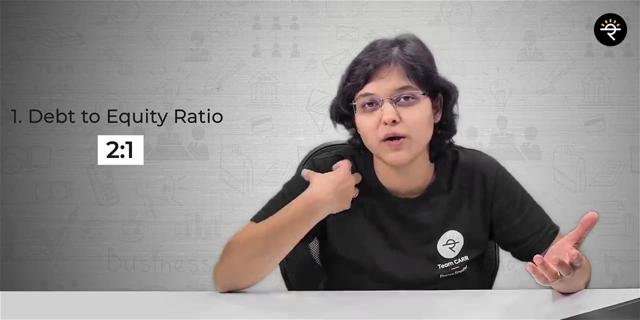 like that. it means that your financial leverage, your- uh, the rate at which you are taking debt, the the total debt i can say is very, very, very high as compared to your own funds. it can be risky when your revenue starts to drop. okay, there could be certain sectors which are. 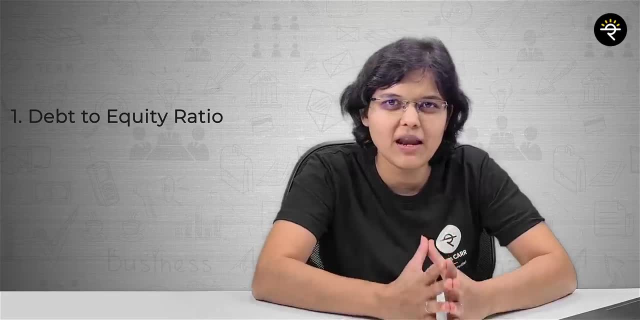 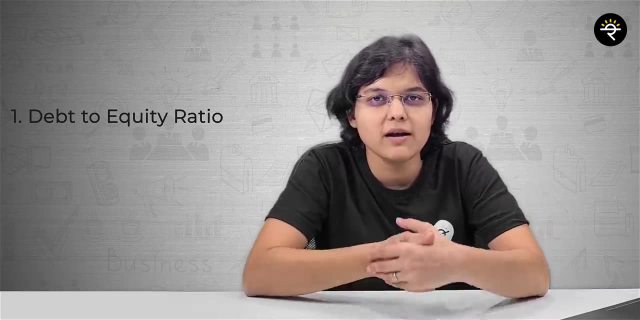 very highly leveraged. one of the example can be real estate, but then if you're not really comfortable, if you are, if you're getting scared, then then you should stay away from sub-sectors, okay. one very important rule again is that never check this debt to equity ratio for banks. 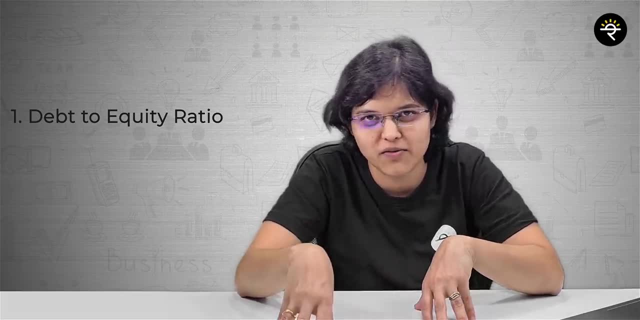 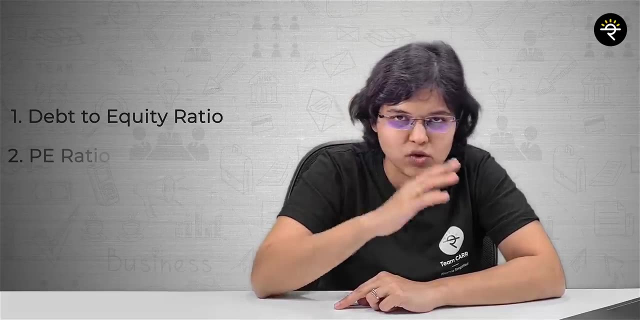 you should never check this debt to equity ratio for banks. you should never check this debt to equity ratio for banks, financial institution as such- because their business model would be completely different. okay, so the first important ratio for you is the debt to equity ratio. second one is your pe ratio. 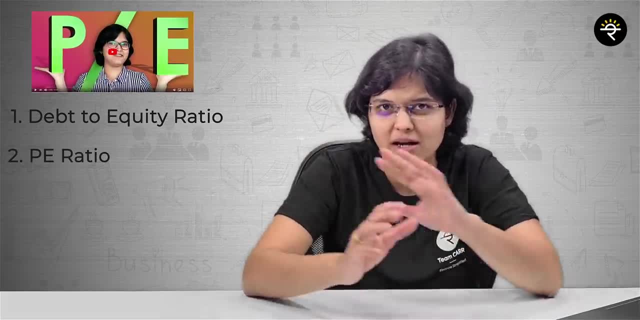 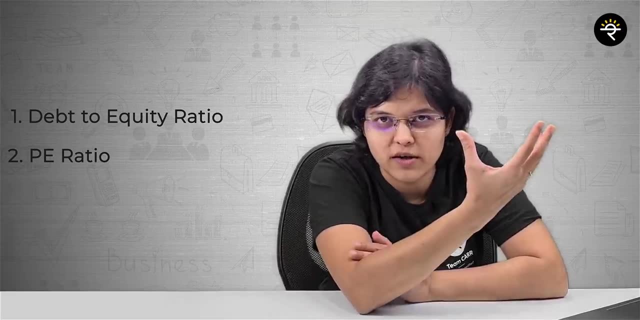 price to earning ratio. i've made a separate video on what is p. the concept has been very well explained in this p ratio basically tells you in simple words how much- uh, cheap or how much pricey the stock is okay. the higher the p, pricier the stock is, lower the p. 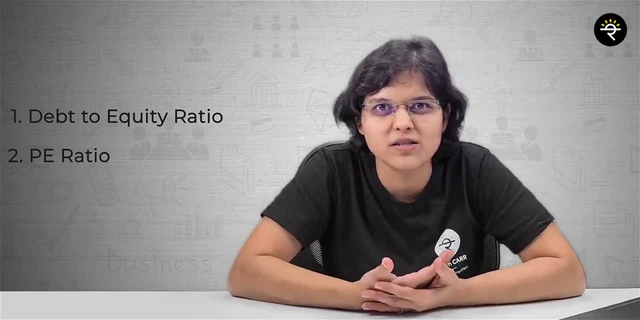 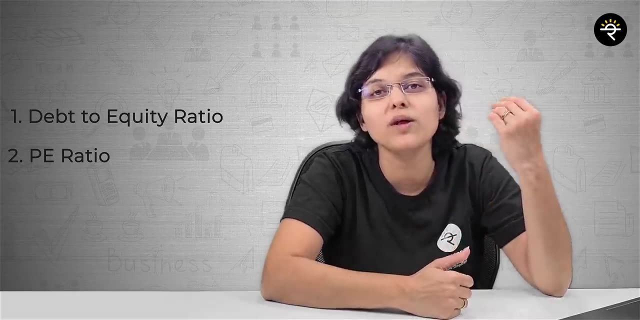 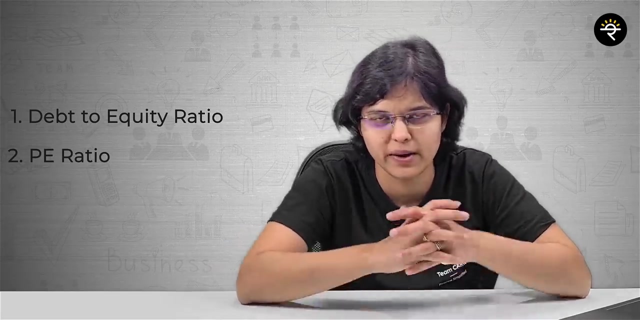 cheaper the stock is, but how can i say like is 20 very expensive? so for that i need to compare the stock pe with the industry p or i can compare the stock pe with another stock p. okay, you can find this data on so many websites. uh, i have covered many websites, even on my channel. so whenever 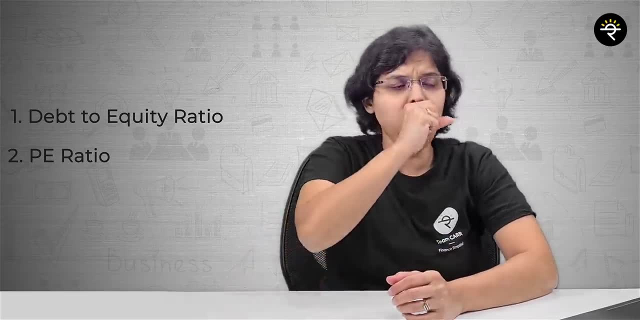 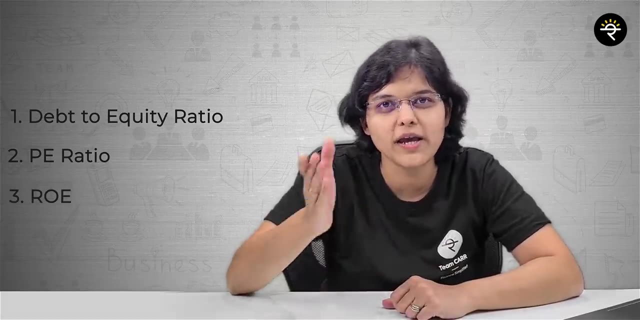 whenever time permits, you can check those as well. right, the third, third stock. i'm sorry, the third ratio that you have to check is the roe, and what is roe return on equity? what does this mean? how much return are you getting? return is how much profit you are getting on the equity ratio. so 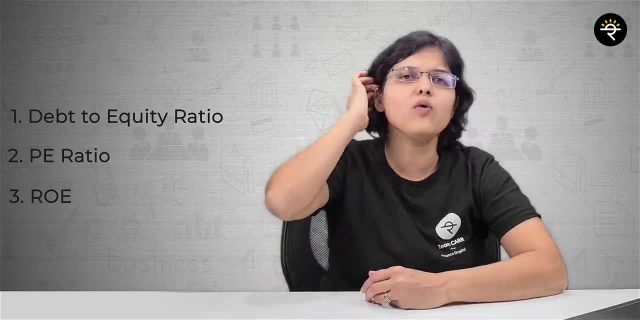 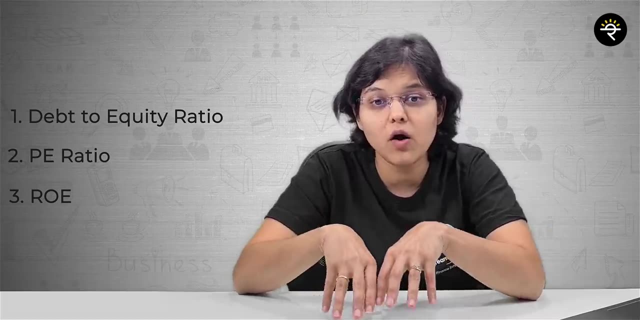 if you are talking about return on equity, you are talking about the equity that has been invested in the business. okay, now how can return be defined? return can be sale. no, can it be profit? not really why? because we are talking about return on equity to the equity shareholders. okay, so if you are from 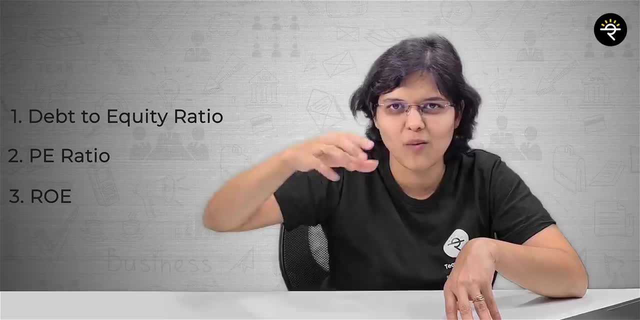 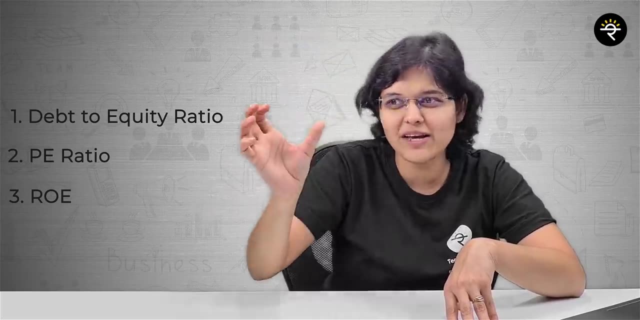 a commerce background, you might very well understand this. first we talk about top line, then we talk about all the expenses. how many other students other than commerce background also understand these basic points if you have been watching my channel regularly? okay, so, top line, all the expenses, then your bottom line is your t80. 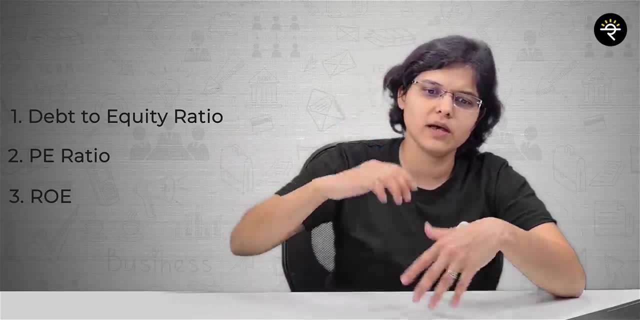 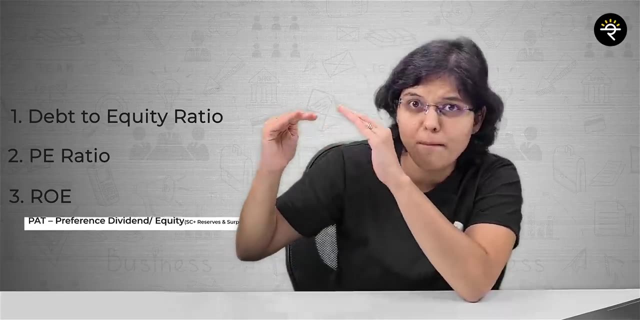 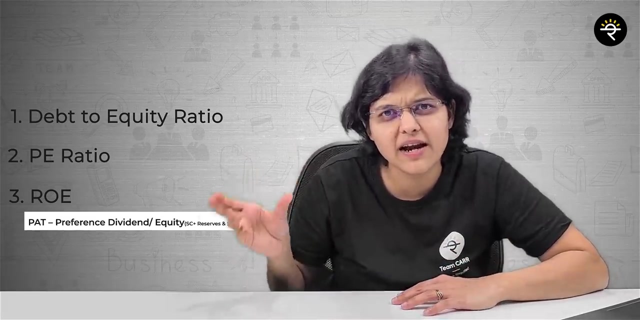 but this p80 profit after tax is- uh, is is, i can say, available for the preference shareholders as well as the equity shareholders. okay, so what we have to do from that? we have to reduce the dividend which is to be paid to the preference shareholders and whatever we get at the end. if, after giving 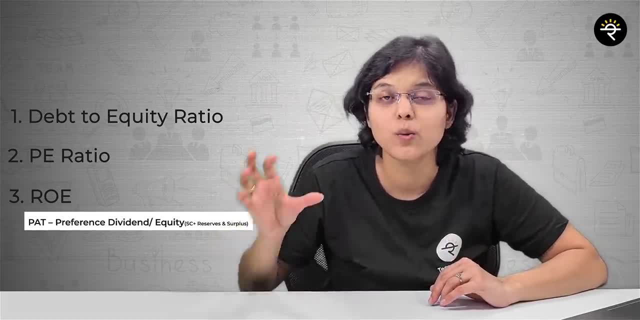 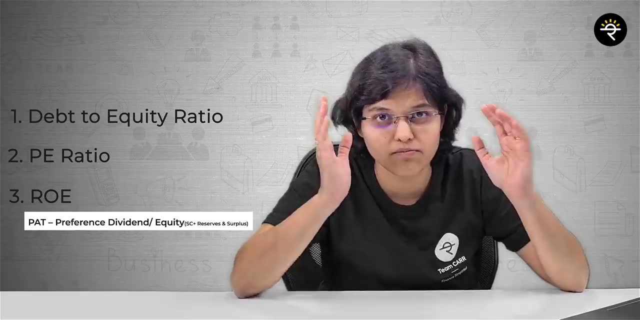 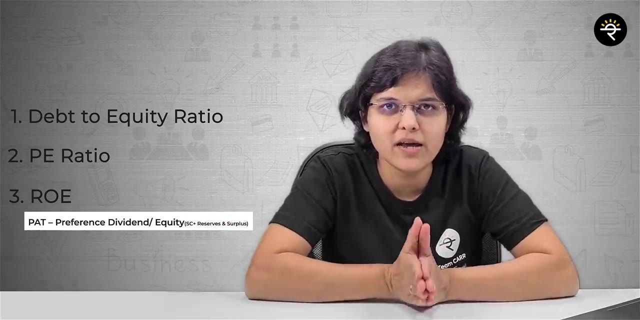 everyone. whatever is left, that is your profit after tax, which is available only for equity shareholders. that amount, when i divide by equity equity, is total equity. so that will be your share capital plus shareholders funds, uh, plus, sorry, reserves and surplus. that will be your shareholders funds. all put together that will give you return on equity. okay, tell me quickly. 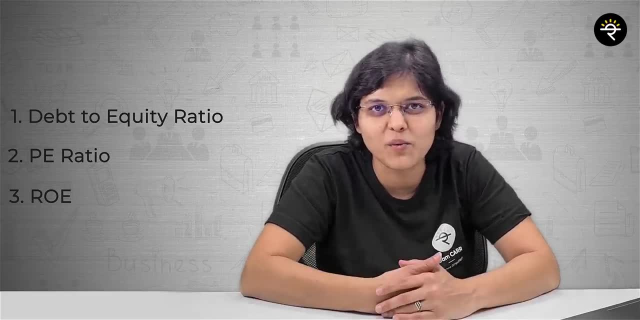 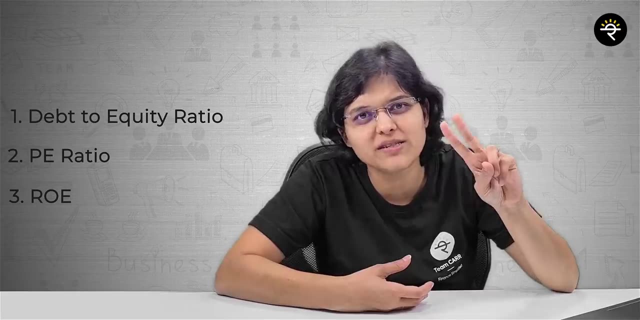 higher the better. lower the better. obviously higher the better. why, if i am generating more return from the business, obviously better it will be. so if i am talking about a business whose ro is like two percent, i would say: just why is the businessman doing the business? better he will. go home better. i think he should just sleep and enjoy. why? because if he is getting two percent better, either do nothing or put your money in saving account. okay, so good. i personally check this out. that roe should be easily above 20 percent, then i take such companies into consideration okay. 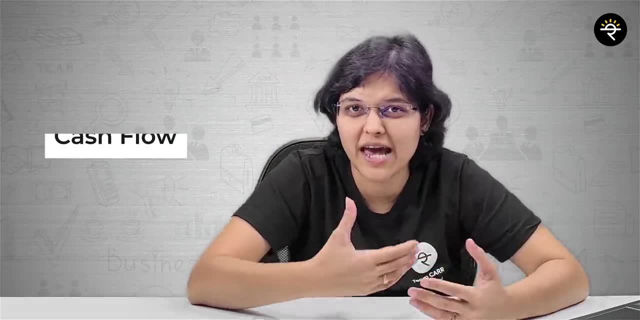 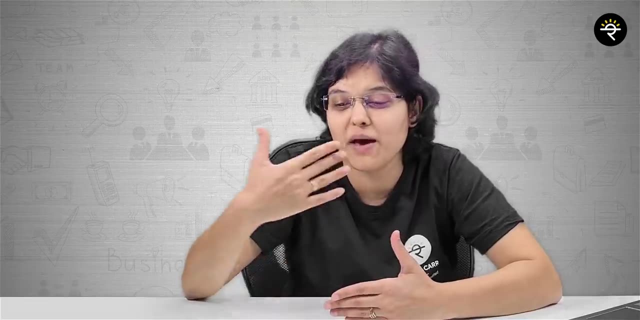 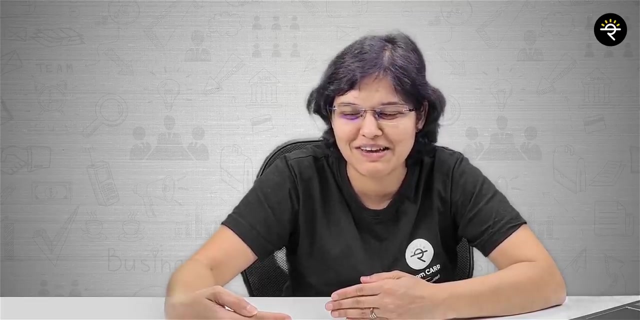 and the third important point that you should be seeing is: how much is the cash flow of the company? it is said that it's it's comparatively easier to manipulate profits, but it's very difficult to manipulate cash flows. very important: i manipulate none in my business, but i'm telling you what certain books say. okay, so going back to a point, which two important cash? 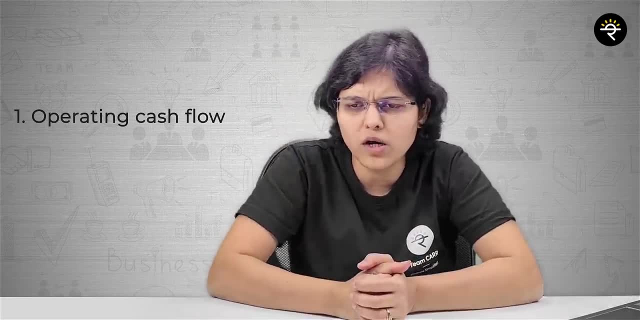 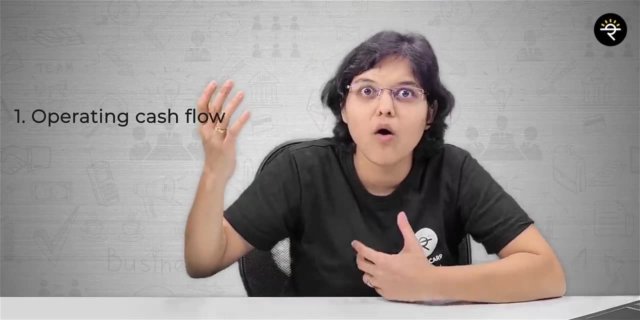 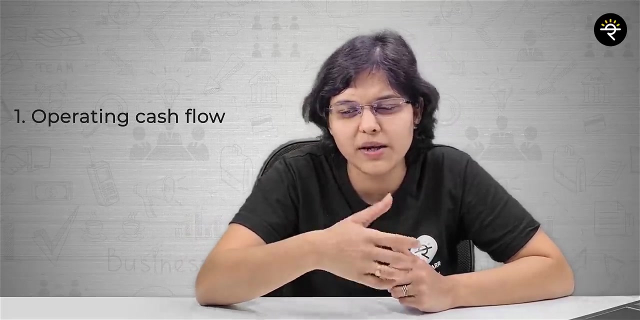 flows you have to analyze. number one is operating cash flows. now, what are operating cash flows? how much cash is being generated from your core business? okay, higher the better. obviously, because more and more your core business is generating, that is always considered to be a positive sign. so whenever you are analyzing a company, check: how much is the last year's operating? uh, how much is?